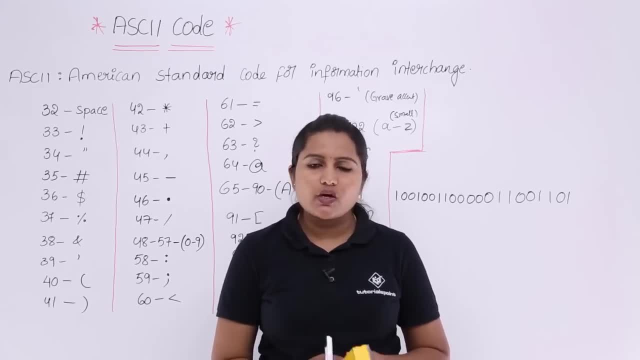 In this video we are going to discuss ASCII code. So ASCII stands for American Standard Code for Information Interchange. So here we are having totally 127 ASCII codes for decimal equivalent. So here for our technical exams I take in some important codes. So rest of you are having in. 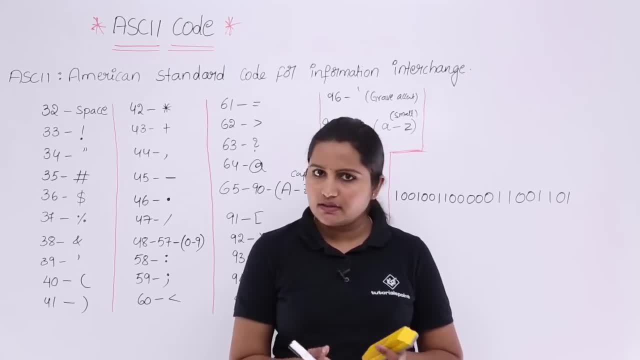 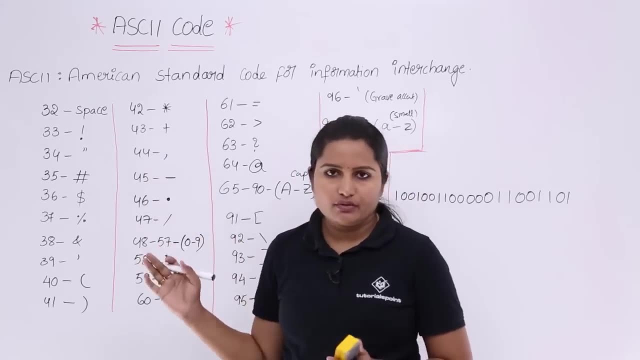 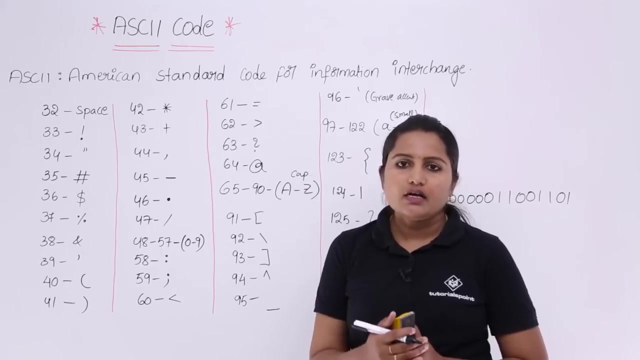 google or you can google it anywhere. you can get you that ASCII chart, So containing all 0 to 127, but so 0 to 31. we do not require much in technical exams and 127 code that is for delete. also we do not require that is of computer short cuts. So all based on these codes you are going to 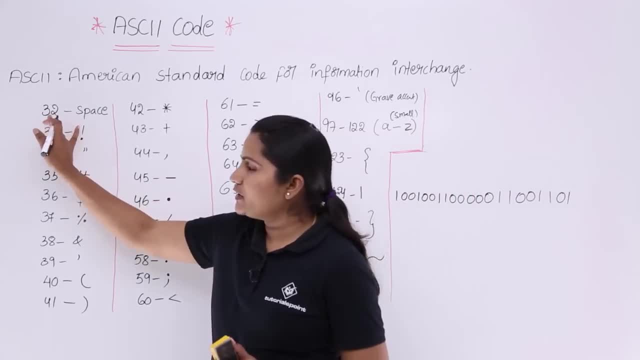 get questions. So now see here: So 32 in decimal will be taken as space in ASCII code, so 33 in decimal. okay, So, and nobody will be told anything else. So 302 in decimal documentation will be taken as space in ASCII codes. So 33 in decimal, you can say. but I am testing that also as 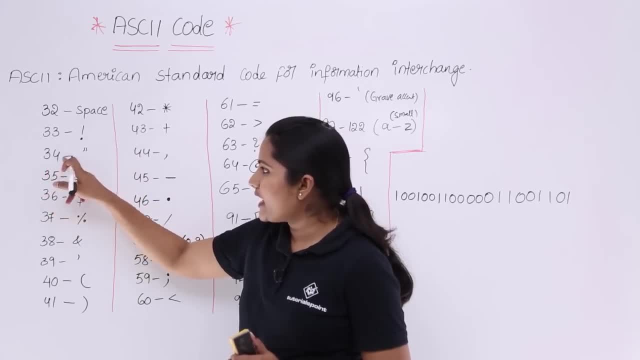 free using elements. So that means this chart cannot be edited and not an issue. WAY gotta say that sook, we is taken as exclamatory mark and 34 as this hyphen and 35 as hash, 36 as dollar, 37 as 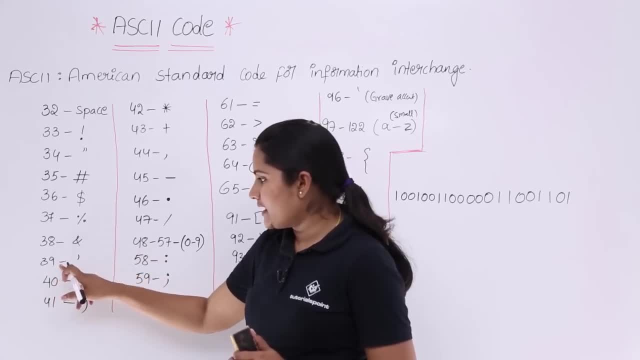 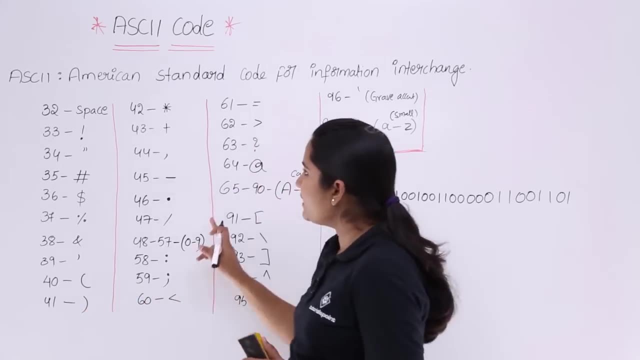 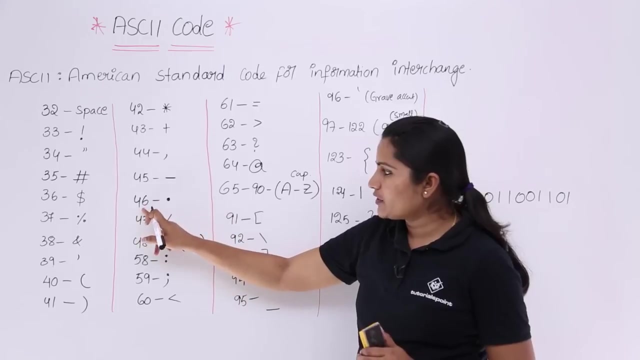 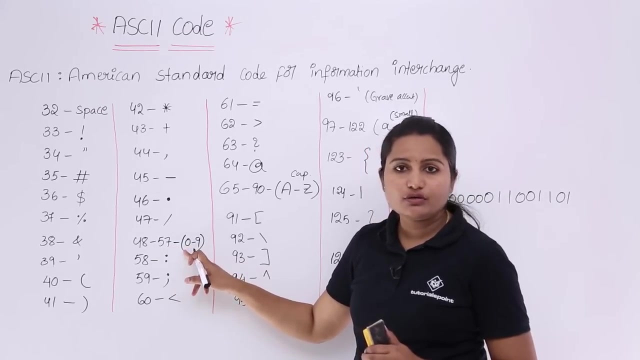 percentage: 38 as end, 39 as single exclamation mark and 40 as open brace, 41 as closed brace, and here 42, asterisk 43 plus 44, comma 45, hyphen 46, dot 47, forward slash 48 to 57, that is 0 to 9. 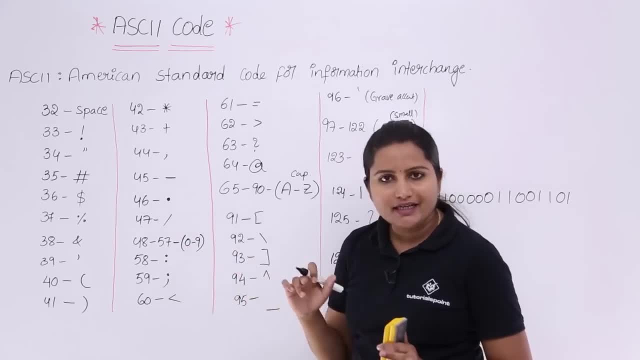 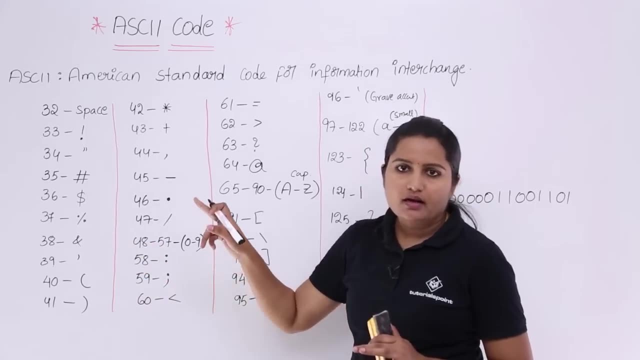 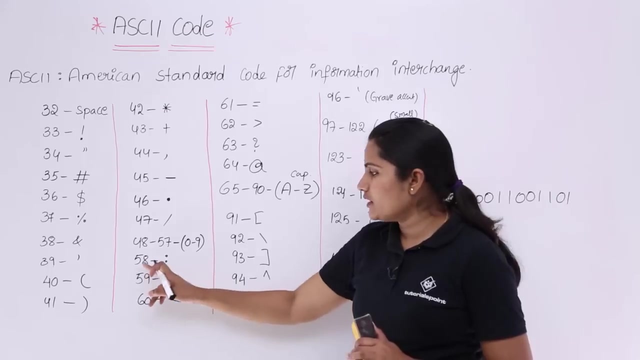 numbers. that means 48 means 0,, 48 in a decimal means 0 in ASCII. So 49. so that means 49 means 1,, 50 means 2, like that 48 to 57. So in 58, so this is colon, so 59, so this is semicolon, and 60 less than and 61 equal. 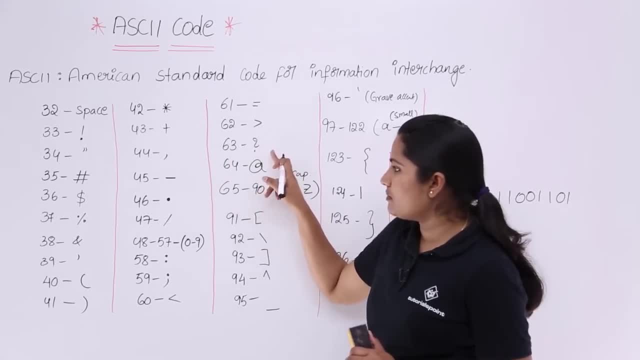 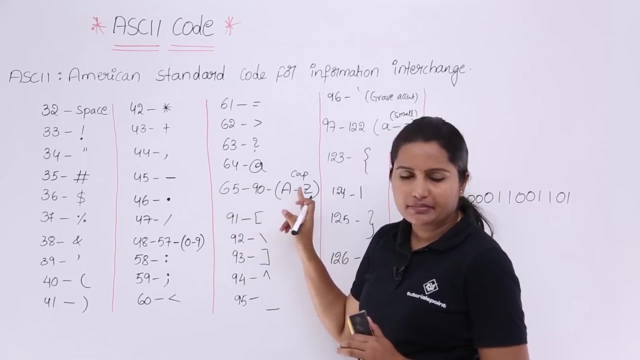 to 62 greater than 63 question mark, 64 at the rate and 65 to 90 uppercase of A to Z. that means capital letters from A to Z. So that means 65 is capital A, 66 is capital B, 67 is capital C, like that. So from 65 to 90 we are having all capital. 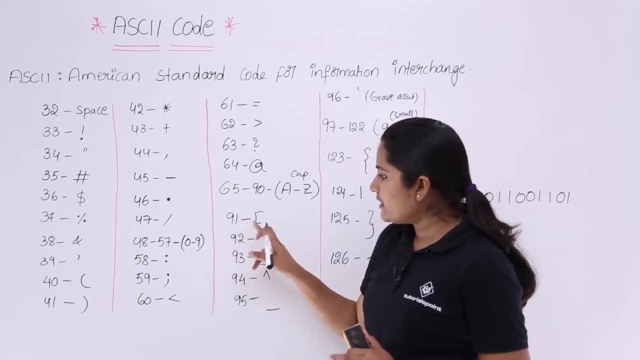 alphabets from A to Z: 91- square bracket- open square bracket. 92, backward slash. 93, closed square bracket, and 94.. So this is somewhat we can say, this is power. So 95, this is underscore, binary, essentially distance from. 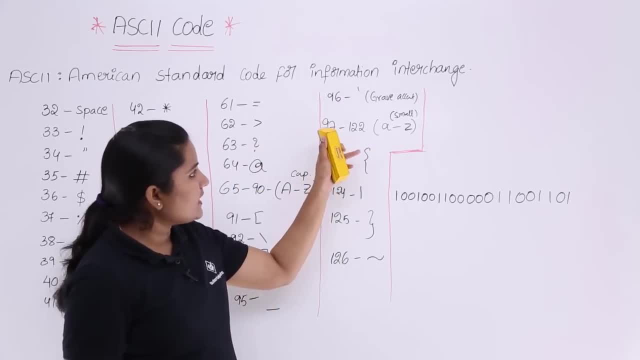 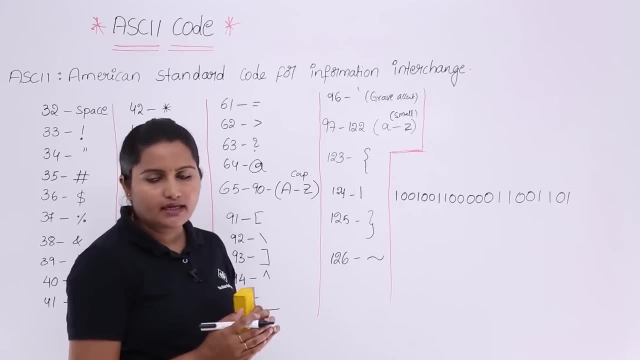 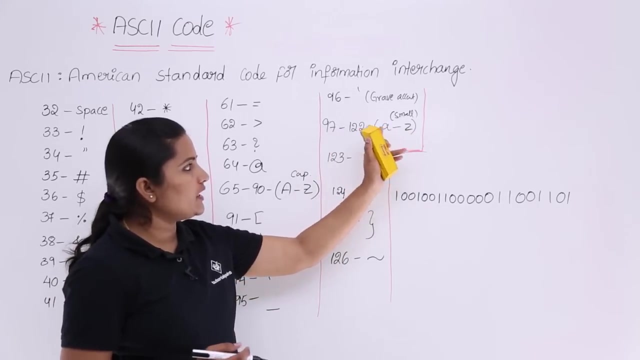 a to q, x less than distance from i to z will not. there will not be difference between 0 and 90,. we are having this feeling of v angle and we are saying this is the thickness of L and z per meters. irritated interior of benzene. Now this is the reconstruction. 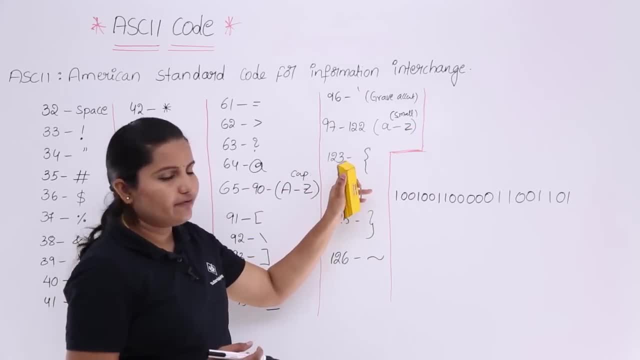 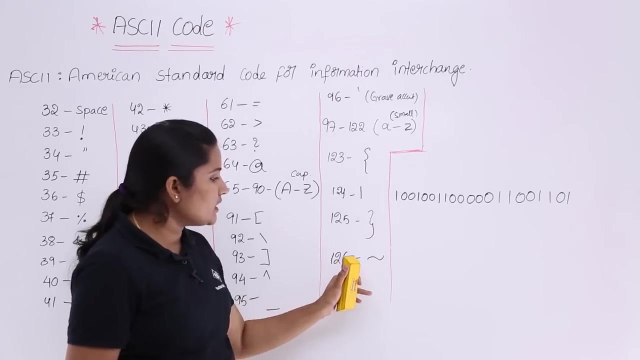 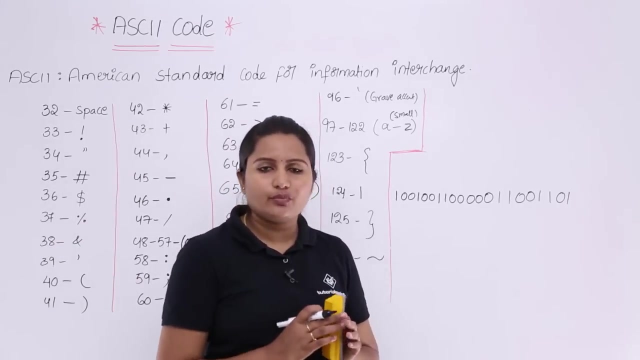 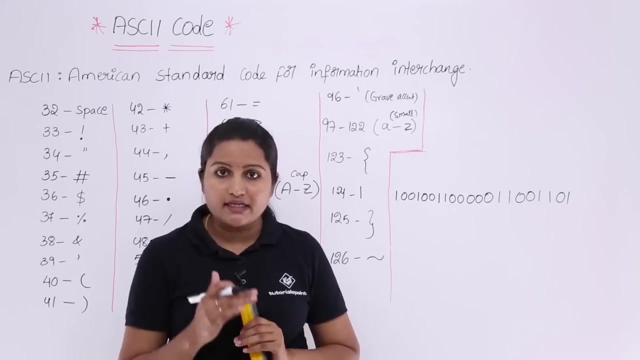 of32 ��고 V, extending from as strike line so, or vertical bar, we can say so. this is not 1, this is vertical bar, 125, closed flower bracket and 126. this is equivalent, nearly equivalent. So now how we are going to get problems in this. ASCII code means ASCII code is generally a 7 bit code, 7 bit character code in. 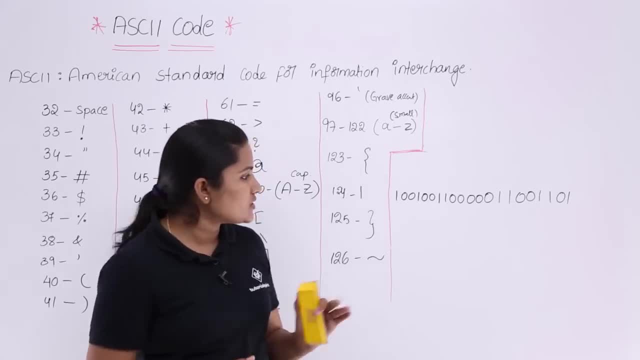 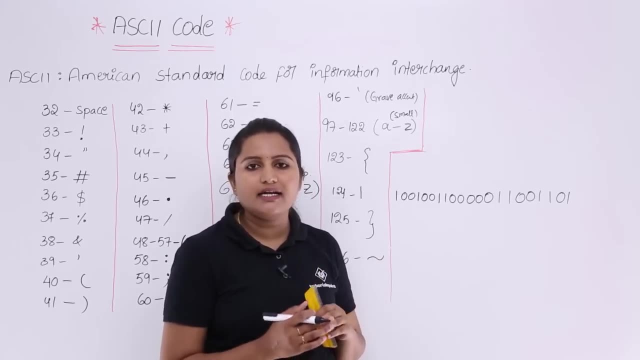 which it includes characters as well as numbers. So see here: for example, this binary data is given in your exams. they are asking: what is the equivalent? what is the equivalent of this binary data? they are asking: First we need to convert this binary into decimal, and then this decimal. 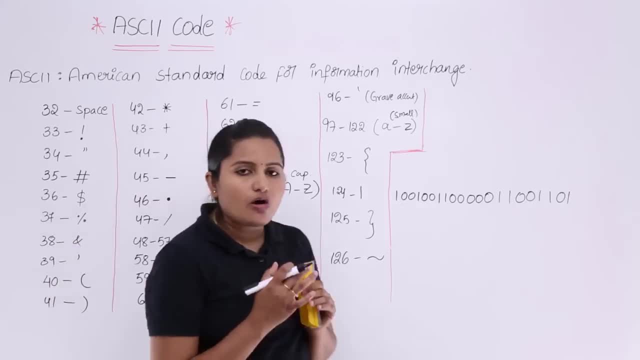 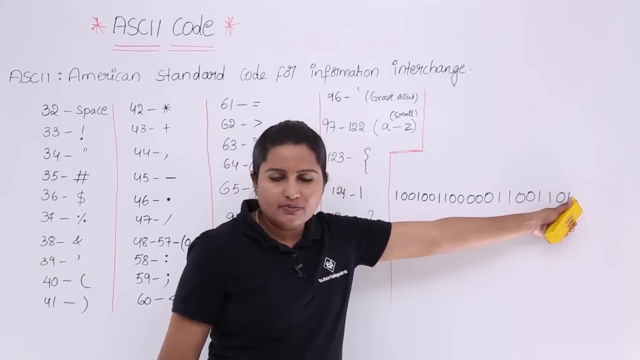 into equivalent ASCII Now. so how many digits we need to group? So in ASCII conversion we need grouping of binary digits. So you know that if you are having any point after digits, then you require right grouping here. you are not having any point- decimal point- then you require only left grouping. 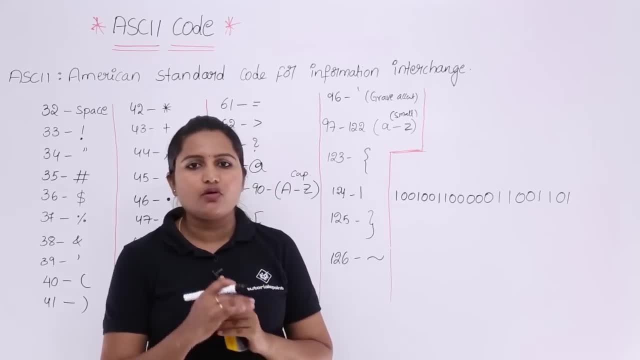 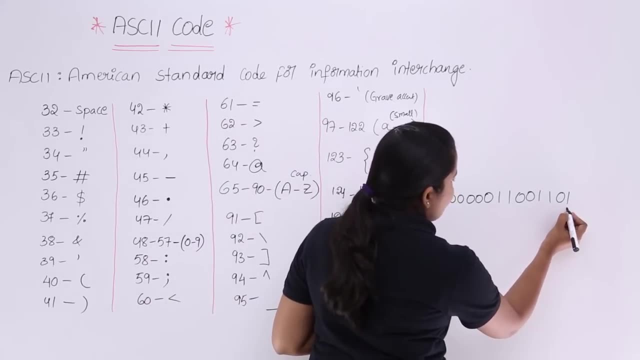 How many bits you need to group means, as ASCII code is a 7 bit code, you need to group 7, 7 bits. So here, see here I am grouping 7, 7 bits. So 7 and another 7 and another 7.. 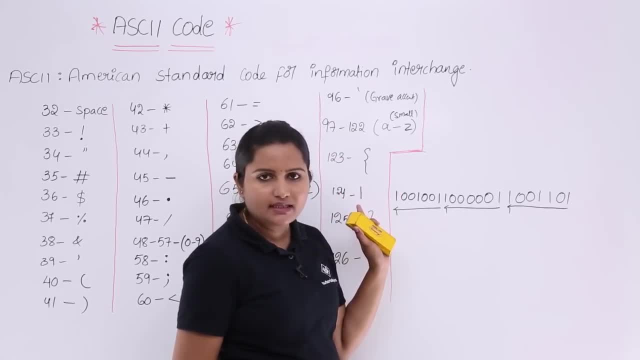 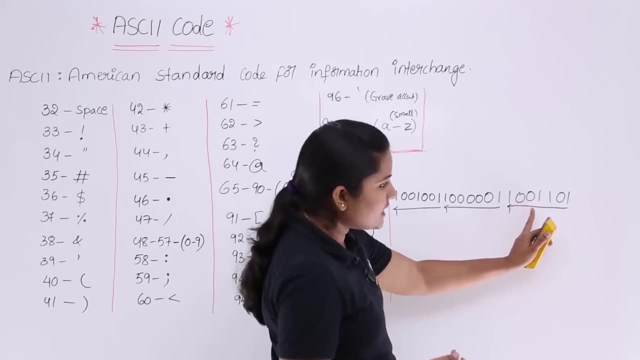 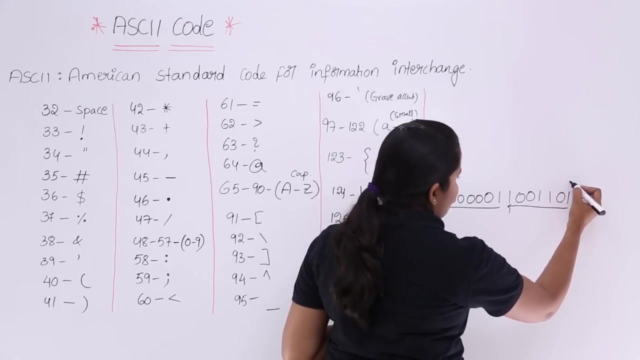 If you are any bits or lack of bits are there, then you can pack zeros. Now see here: So this is the value equivalent to. So if you want to see this equivalent value, you can place values of two powers here. So that means so: 0, 1, 2, 4, 8, and after that 16, 30 to 64. So like this you can see the. 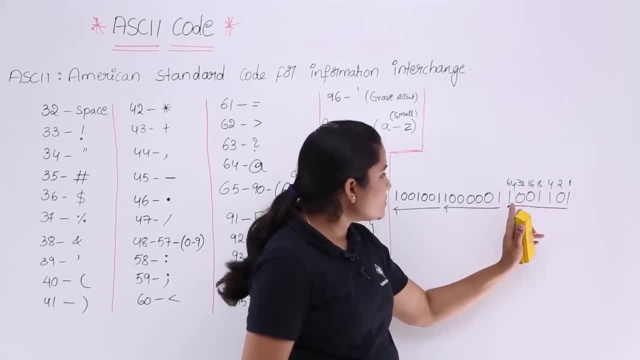 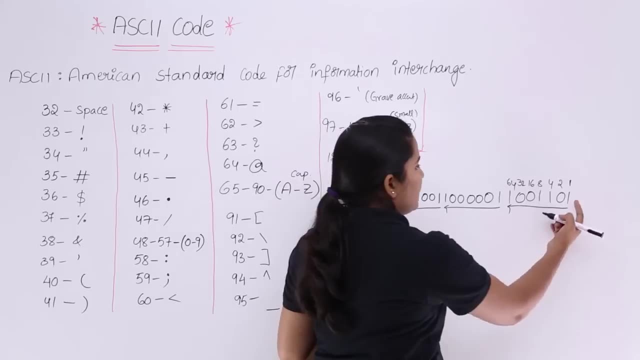 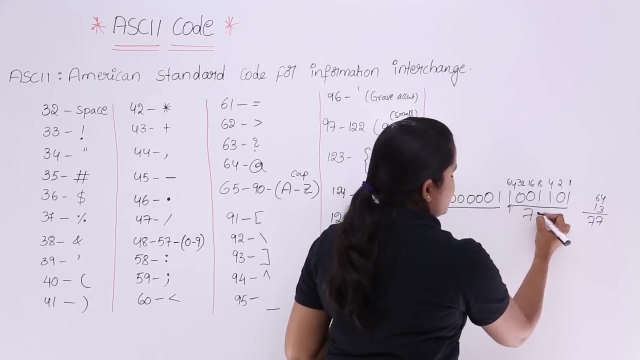 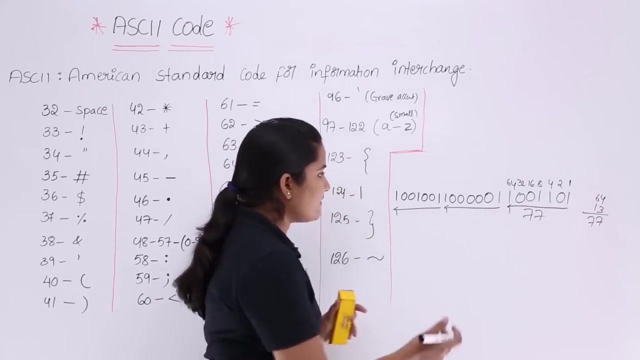 binary or a decimal that is the equivalent of this binary. So 64 plus 8 plus 4 plus 1.. That means this is 13 and 64, 64 plus so 13, you are going to get 77. So this is 77. So 64 plus 13 equivalent to 77. and here this is: 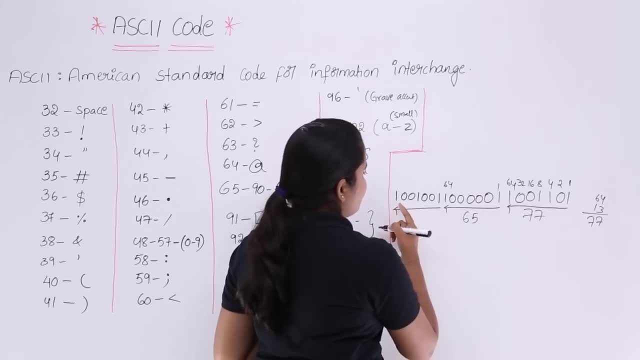 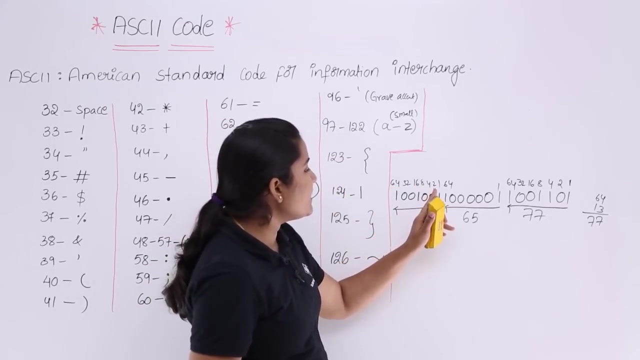 equivalent to 64 plus 1.. So 65, and this is transport officer's value inder associate. So this這樣 is so: 64, 32, 16, 8, 4, 2, 1. so 64 plus 16, you are going to get nearly 80, 80 plus. here you are having. 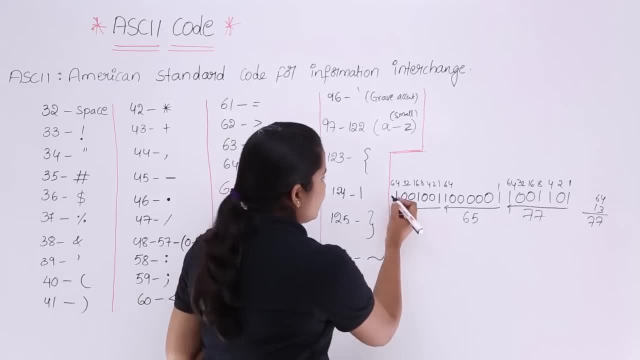 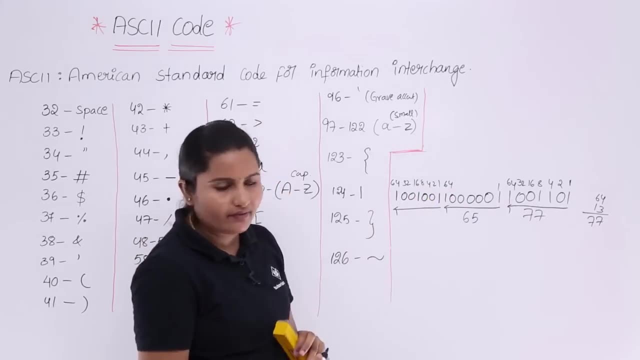 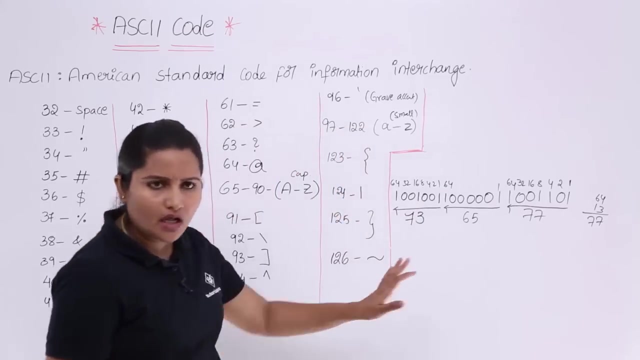 1, that means 81, nearly so here, sorry, this is 8, 64 plus 8 plus 1, you are having, so now 64 plus 8 plus 1 means so 64 plus 8. you are having 72, 72 plus 1, 73, so this is 73 now you converted. 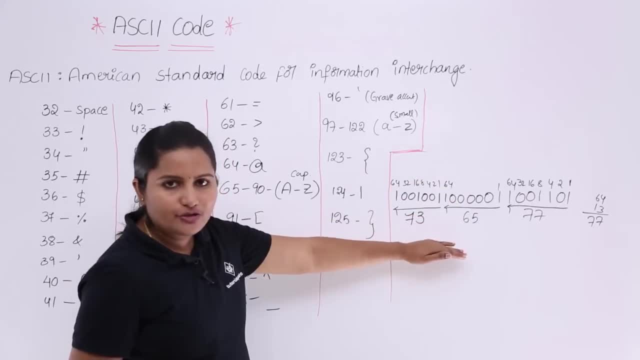 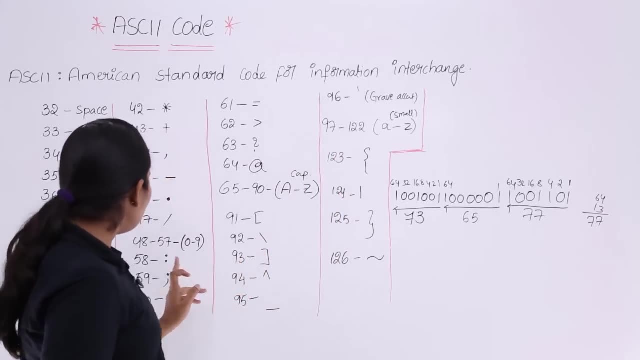 into decimal. so you converted binary into decimal. from this decimal you converted, you can convert into ASCII, as you know that 73 is in the range of. here you can see: 73 is capital letters, capital alphabets, 73 in the range of capital alphabets, so 73 is equivalent to i, so 73 is. 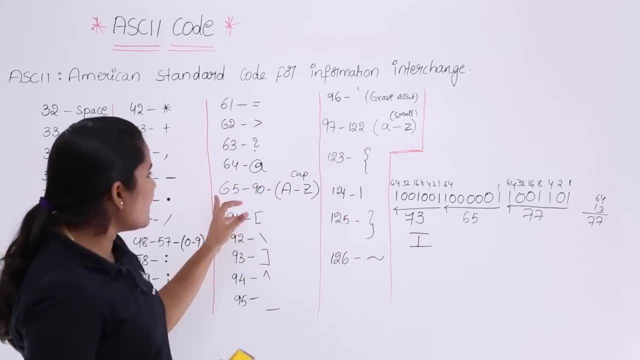 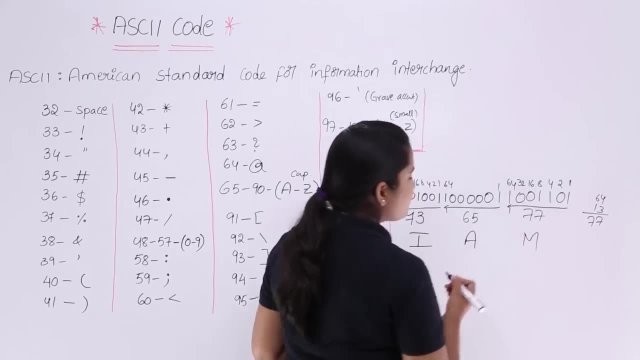 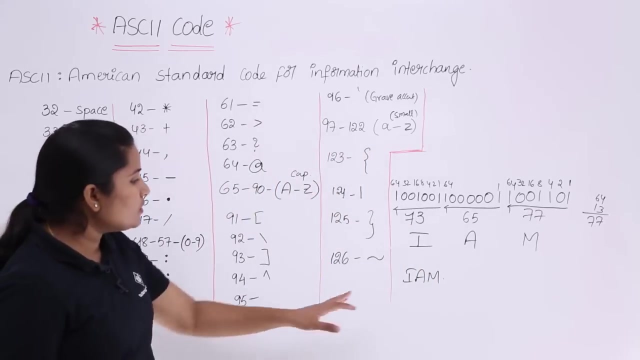 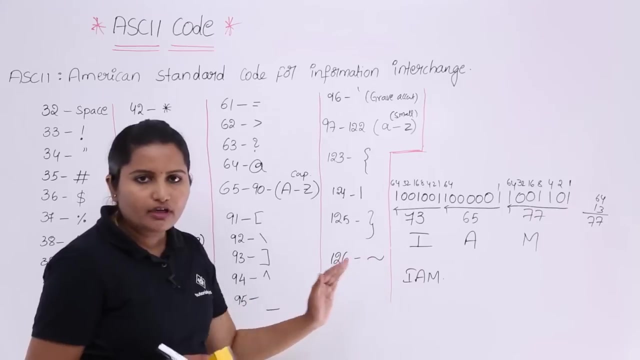 equivalent to capital i and 65 is equivalent to capital a and 77 is equivalent to m. so i a, m is your ASCII code. so now, for example, if you are, if you want any space in between these two, you need to consider space or hyphen. 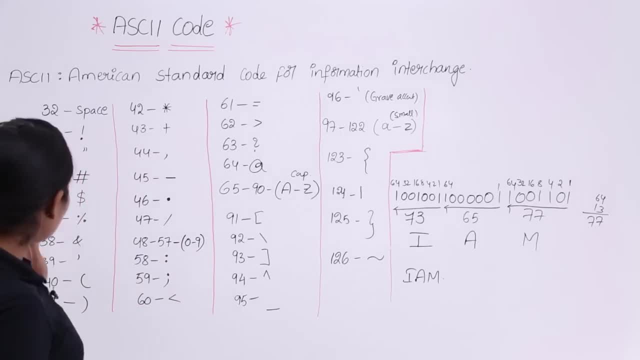 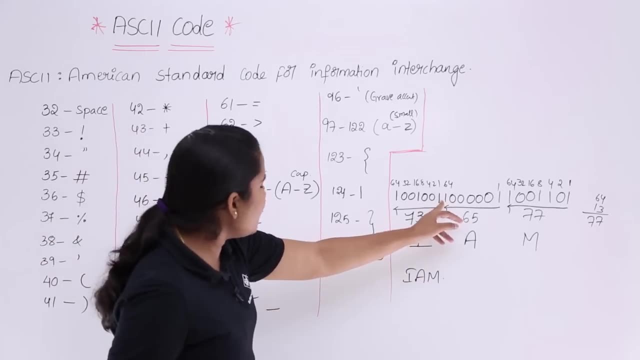 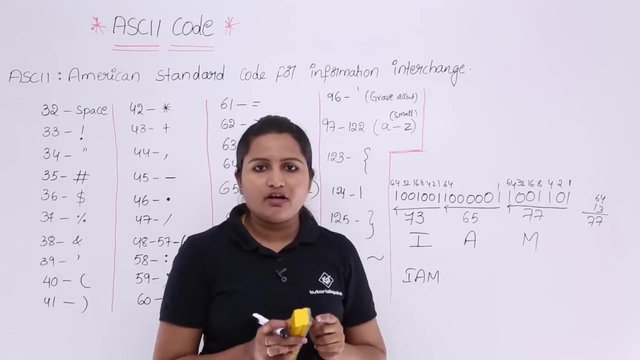 for this. that means, for example, if you require any comma or if you require any hyphen in between i and m, so here you need to include some 45 or anything, or you need to include the value equivalent to space that you can get in the chart of ASCII. 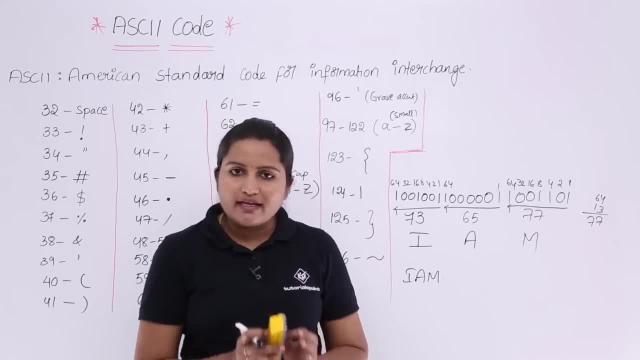 Thank you. So this is about ASCII code. so whenever you given with a binary data to convert into ASCII, definitely you need to get grouping of digits. 7, 7 bits you need to group. if is there any lack of digits you can pad the digits. so grouping is as usual. in other cases, like hexadecimal and